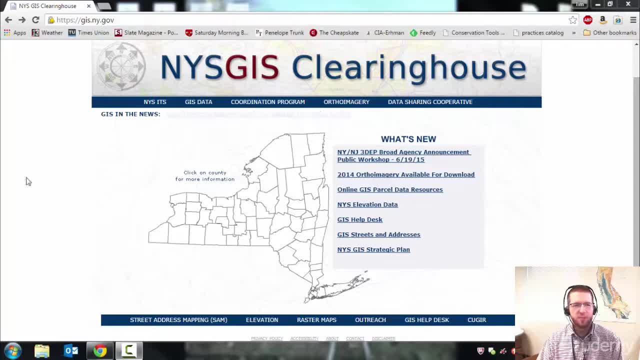 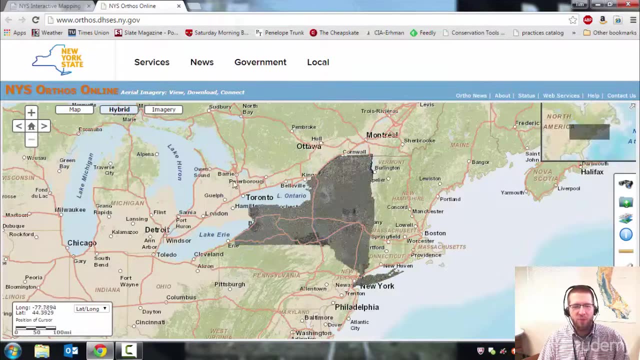 working in a soil and water district in New York. So just browse to that, if not just google search it. Once you're on the home page, you click on the ortho imagery link here and then start the ortho imagery application, And this is their kind of a web map portal where you go to download. 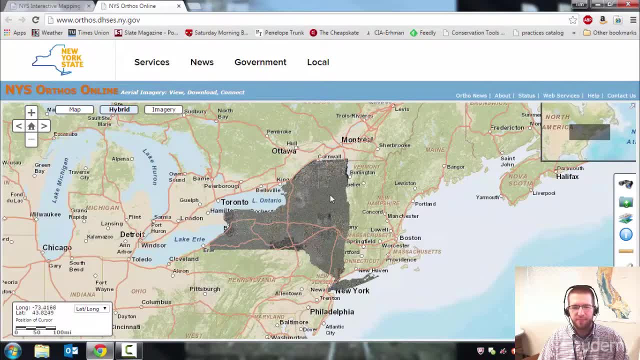 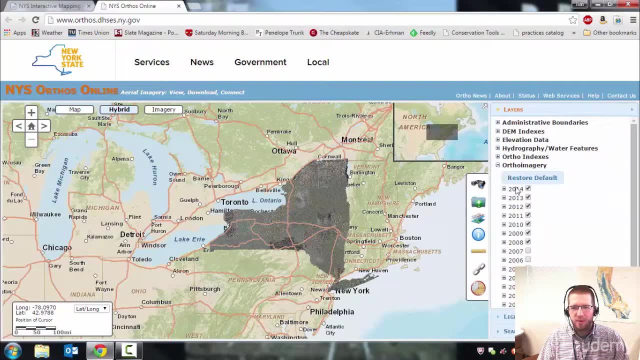 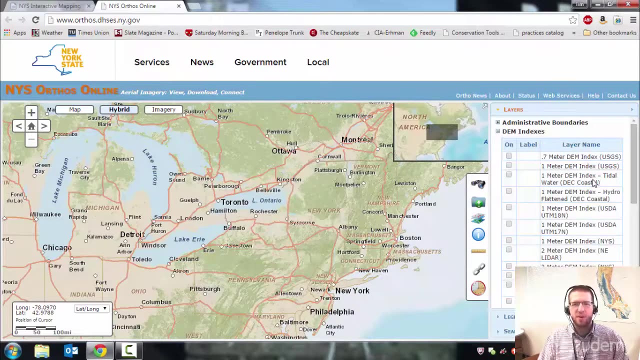 aerial photos. if you want to use those in GIS, First click over on the layers button over on the right and let's turn off all those orthos. That'll let us see what DEMs are available better. So the lidars are stored as DEMs. That's a digital elevation model. You see these, all these different. 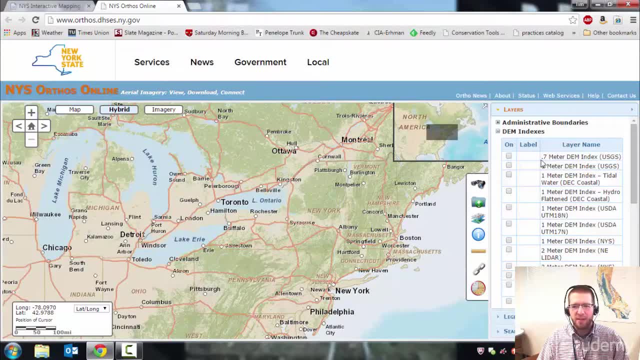 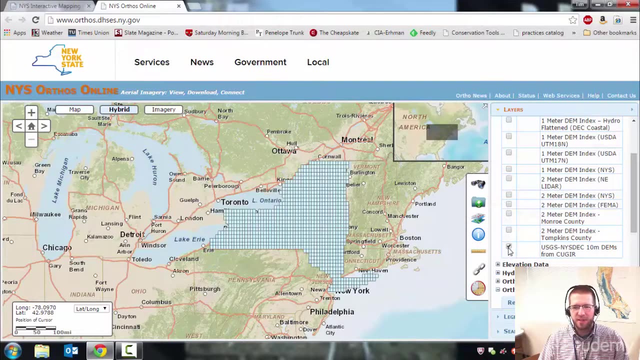 options all the way from 0.7 meter resolution. That's the distance between points in the grid, So a smaller meter number means it's more accurate: 0.7 meter all the way up to 10 meter. Now, these 10 meter DEMs are just derivations of USGS contour maps. They've been scanned in and 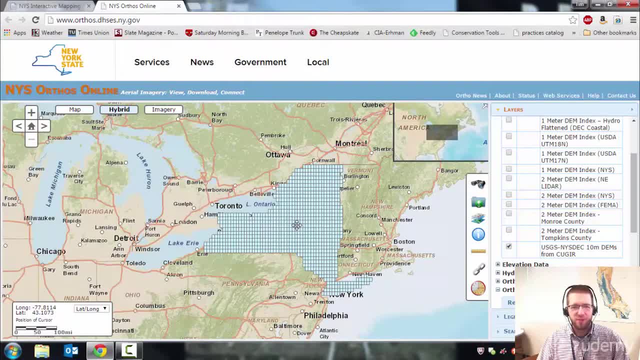 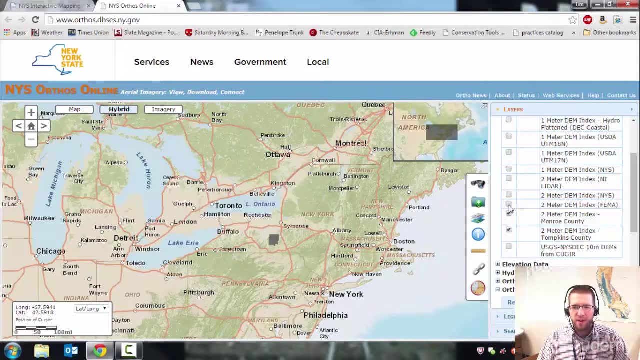 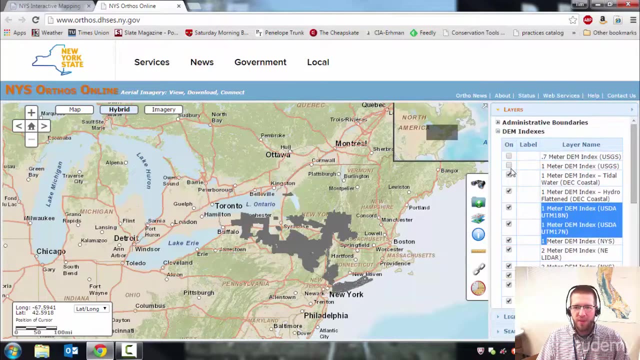 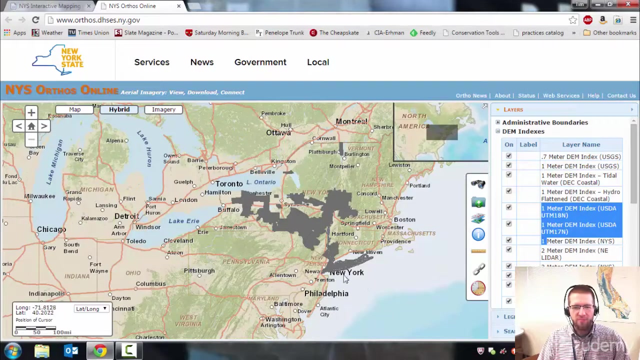 digitized, So they're no better resolution than the contour maps, even though they are digital. So let's turn that off and turn off, turn on all the other ones. And all these other ones are derived from lidar scans. So if you're trying to get an idea of what's our overall coverage in New York for lidar, 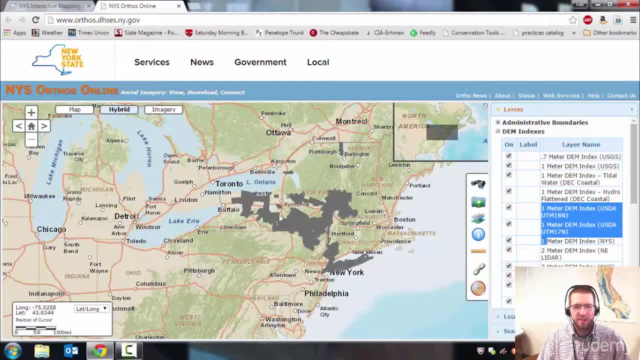 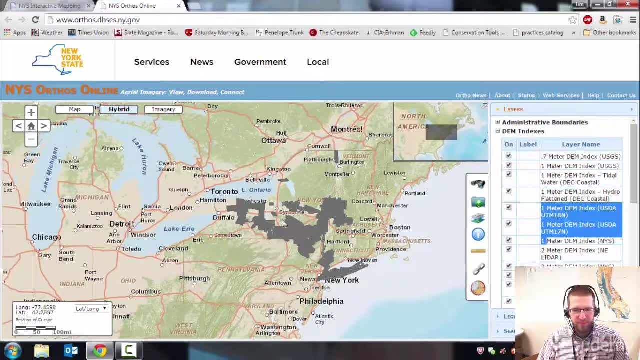 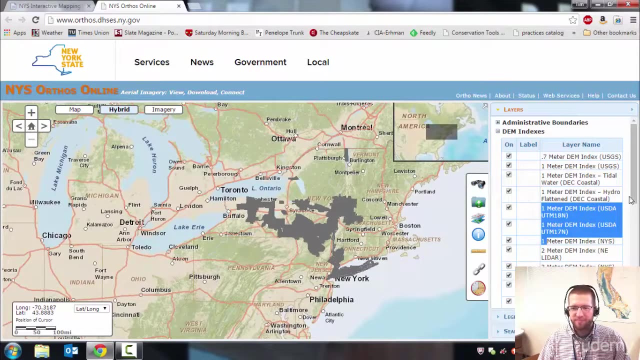 this is basically it. It's all Long Island and you know some southern tier and then kind of scattered counties in between and around. So hopefully you're in a county that has lidar coverage. If not, then you don't get. don't get to use it, All right. so let's look at how to download. 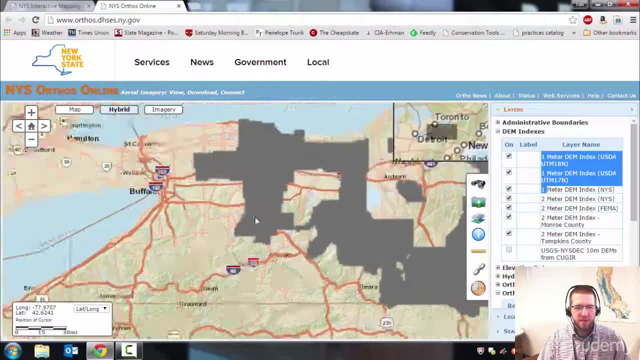 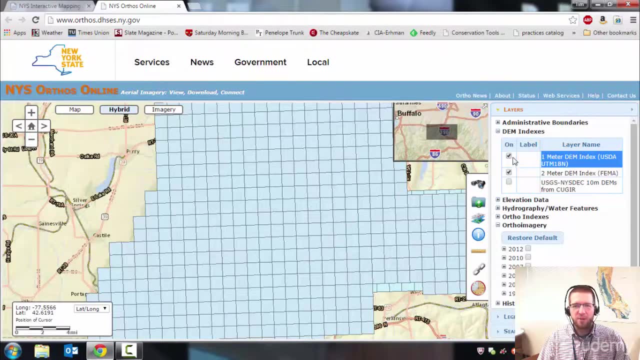 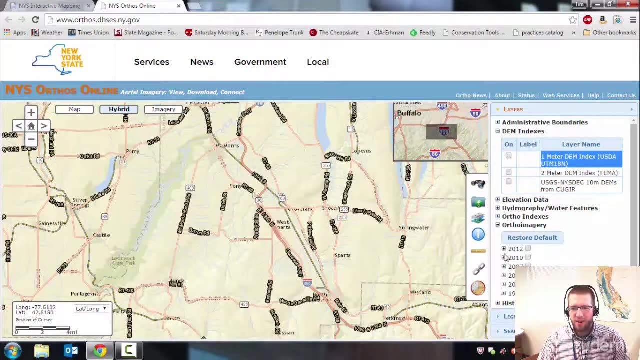 it now Say: we're over here in Livingston. As you zoom in, it'll limit your layers to the only the ones available in that view. So that's kind of nice. I'm going to turn them off off for now and find a farm.